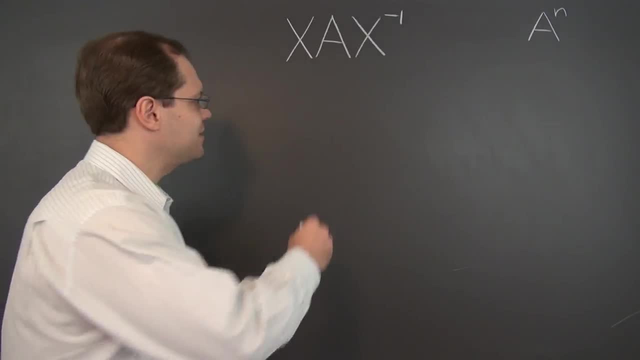 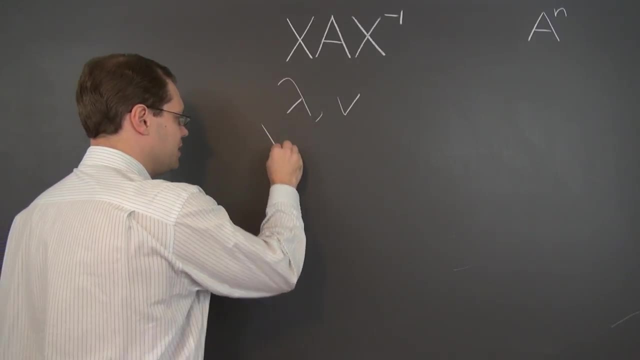 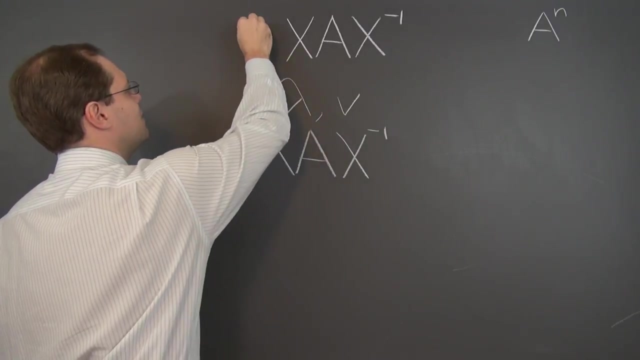 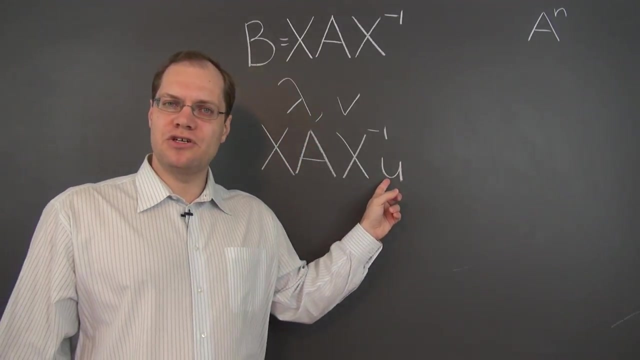 its properties. Suppose that lambda is an eigenvalue of A and that V is the corresponding eigenvector. I will now multiply our new matrix, X A, X inverse. let's give it a name, let's call it B- by a vector, U. And of course I want the vector U to be such that X inverse U is V. Why is? 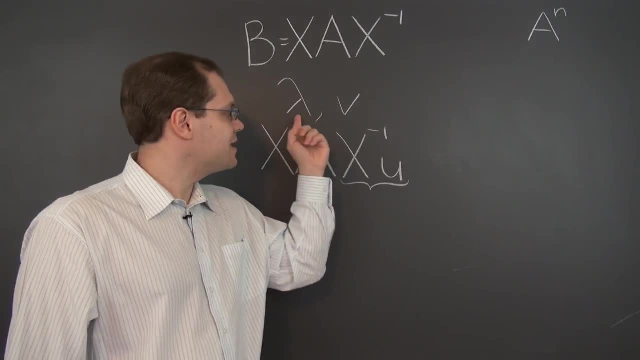 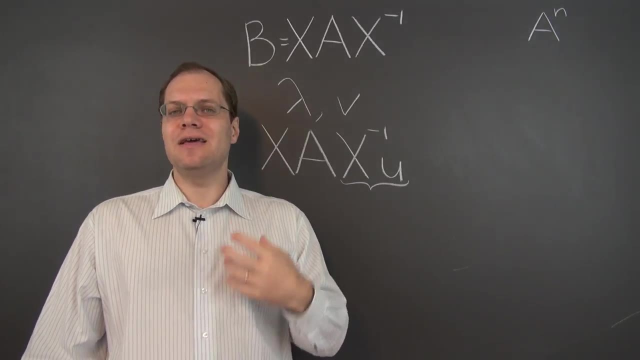 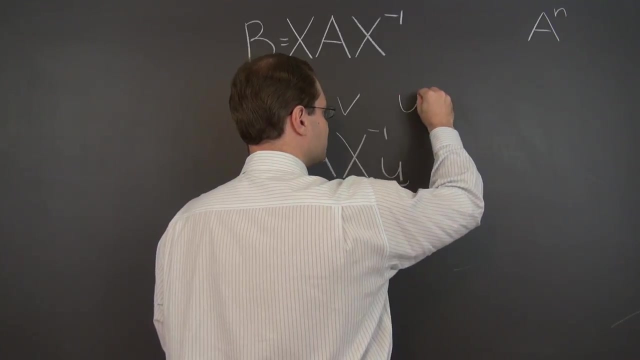 that. Well, because I want to take advantage of my knowledge of eigenvalues and eigenvectors of the matrix A. and if A multiplies V, then I know that A V equals lambda V, which is taking advantage of the only thing I know about A. So I want U to equal X V If U equals. 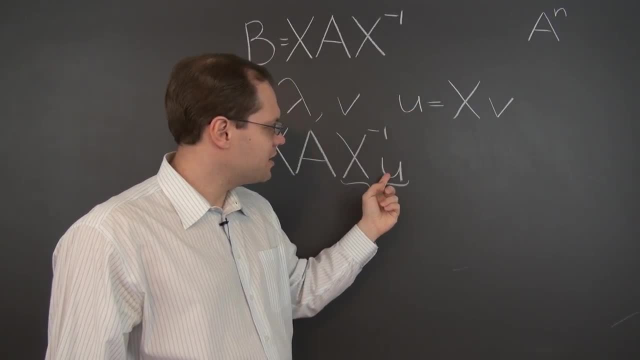 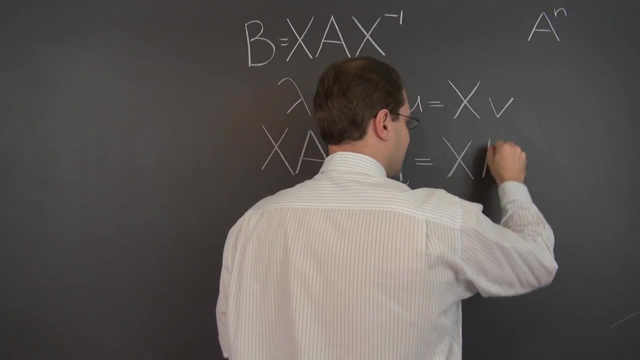 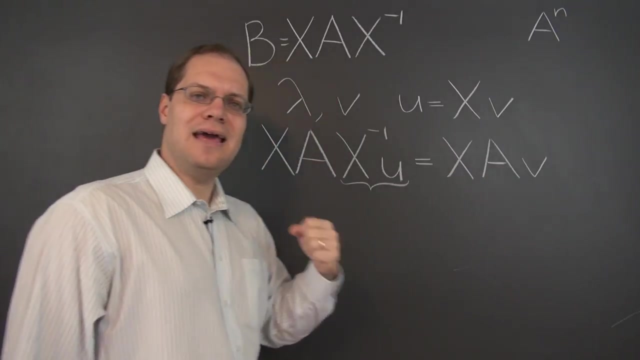 X, V, then X inverse U. what we have here is V, Just what I want. So let's see what we have. We have X, A V, So now I've gotten what I wanted, which is A V. A V is lambda V So. 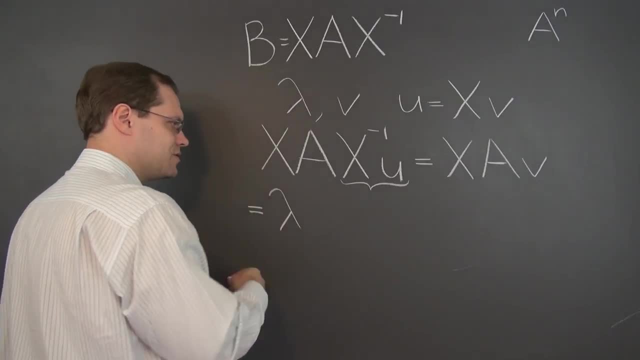 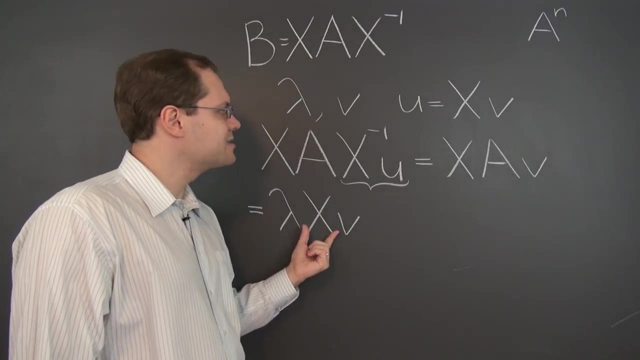 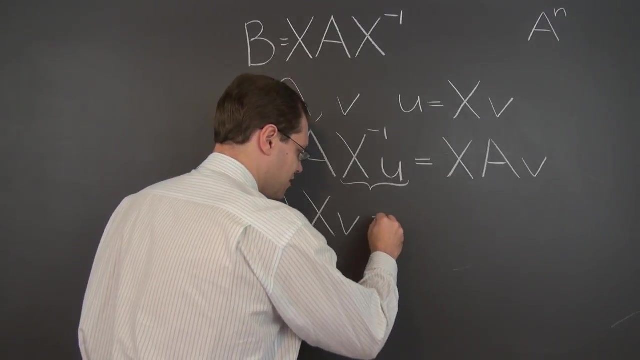 the whole product becomes lambda. It's a number, so it comes all the way out X V. So I got V back and it's next to X and I know what X V is. X V is U, So the whole expression. 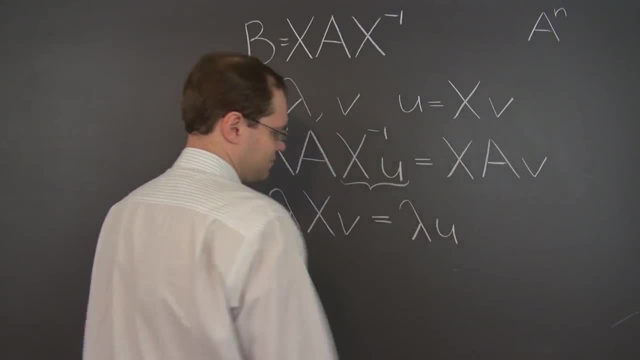 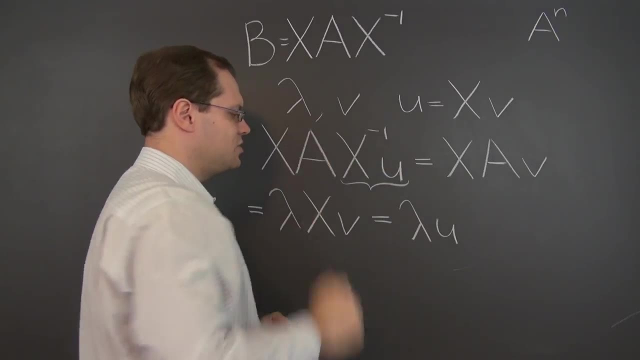 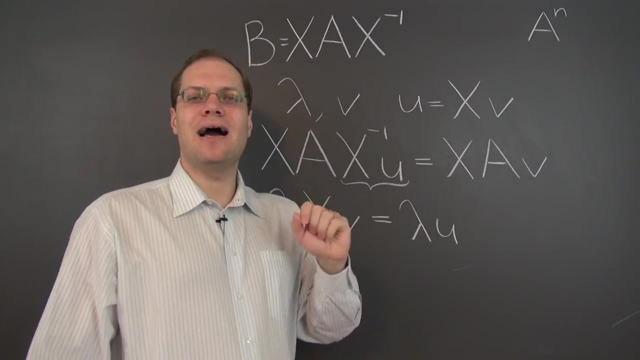 U equals lambda U. So now let's see what we have on the board. What we have on the board is that this matrix, B times U, equals lambda U. So what's the only conclusion that we can reach? That lambda is the eigenvalue of B. B is related to A by the similarity. 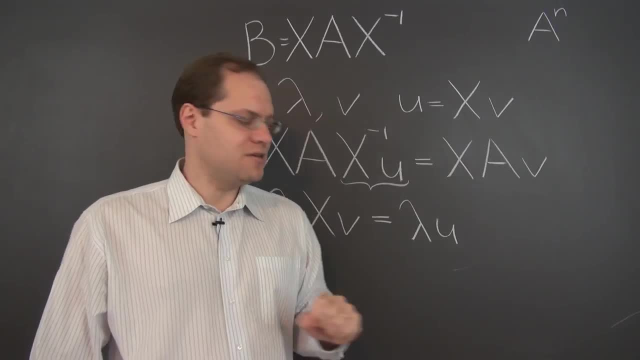 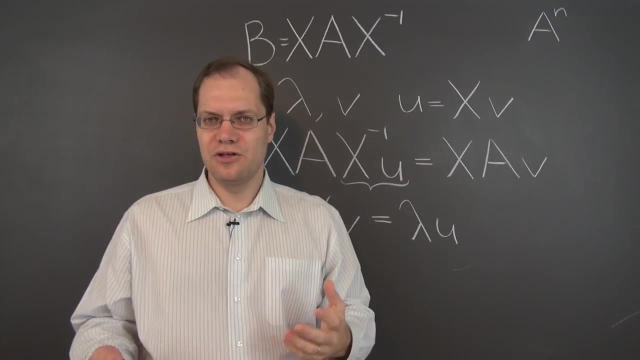 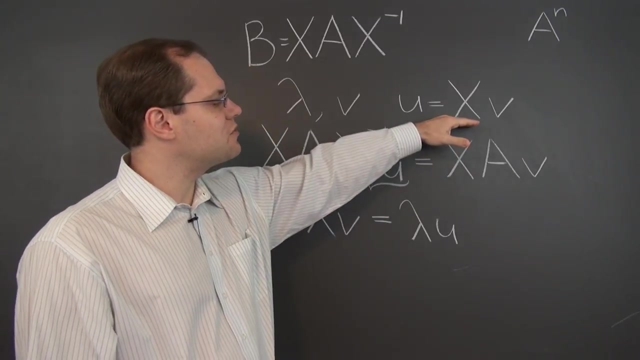 transformation and U is the corresponding eigenvector. In fact, U is related to V by this transformation. So we conclude that A and B have identical eigenvalues and their eigenvectors are related by the transformation X. And do you see how I use the terms matrix and transformation?